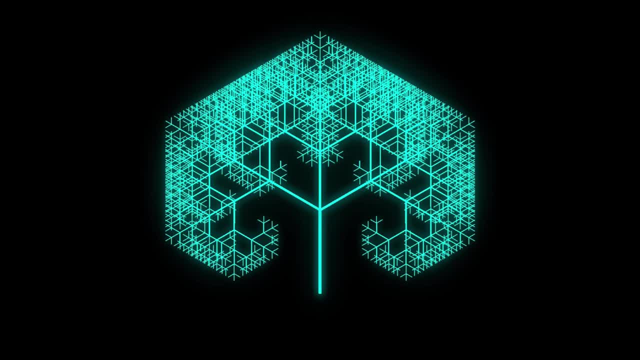 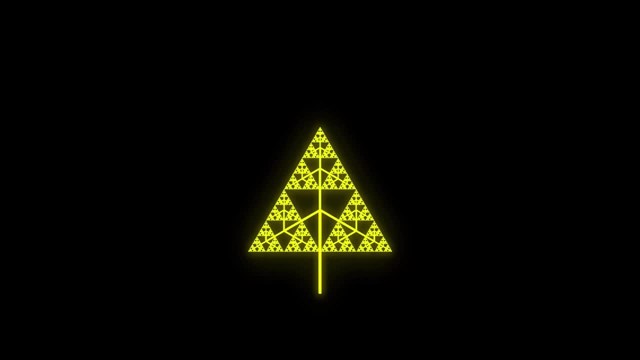 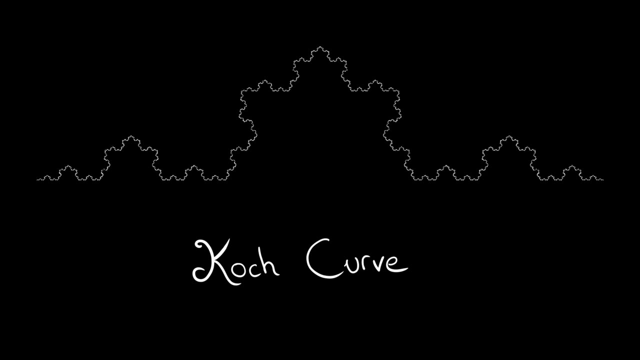 effect and apply shaders. as you'll see later Afterwards, I created a bunch of fractals using Lindemeyer's system. I was inspired by Godot's awesome video on the subject. A link is in the description. I recommend you to check it out. 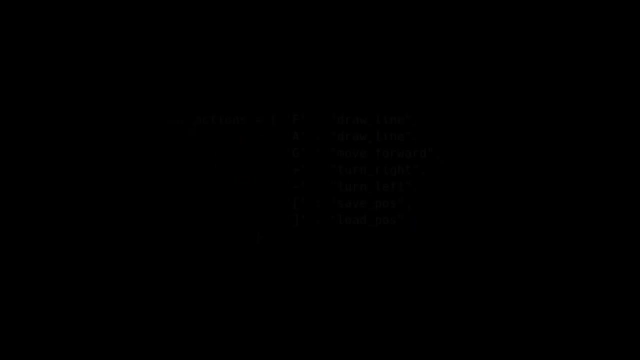 Once I had the grammar functions and some actions to draw the result implemented, it was possible to create a variety of fractals giving an action, which is the really first actions of the fractals, some rules to expand the fractal at each iteration and eventually, 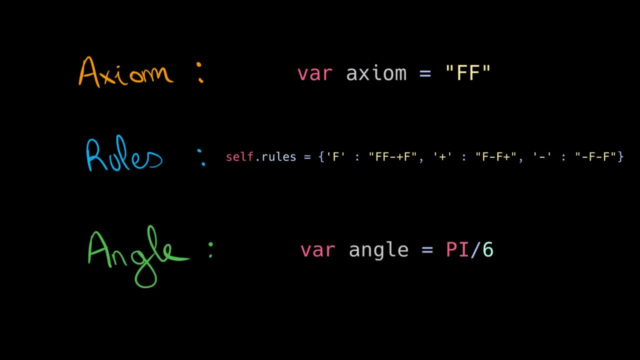 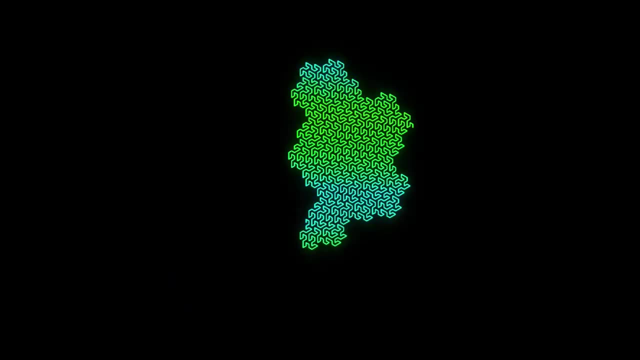 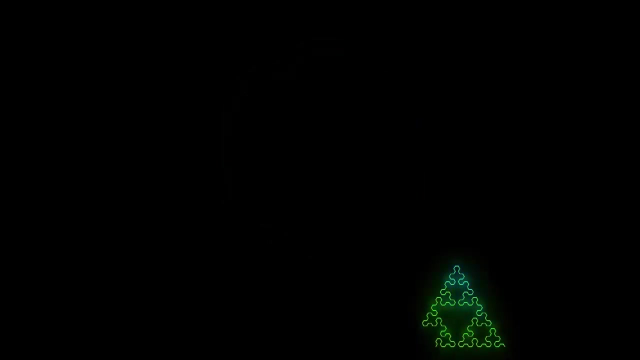 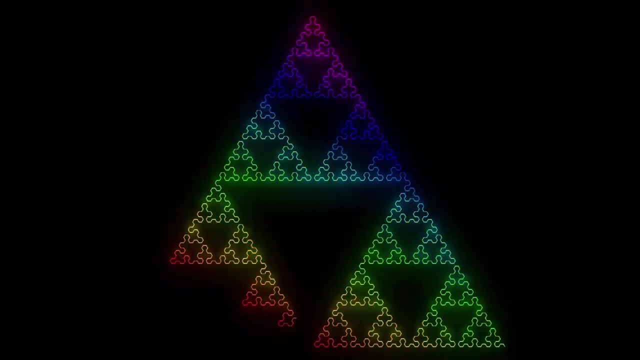 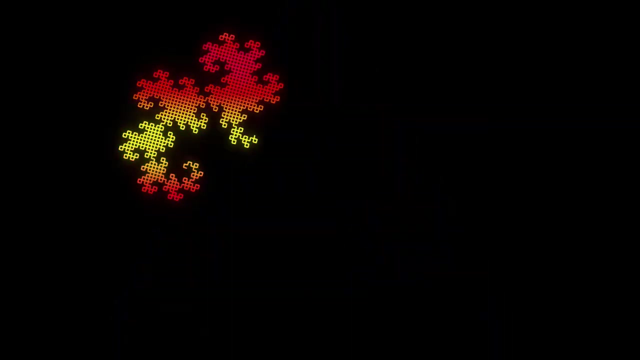 a modification of the angle applied at each rotation. Sit back, relax and watch this with cool music. Take a look: You're listening to Lindemeyer's system and learning how to draw a fractal using the 1D node Like this: 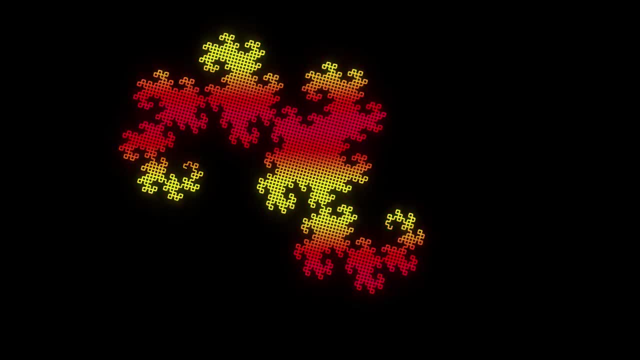 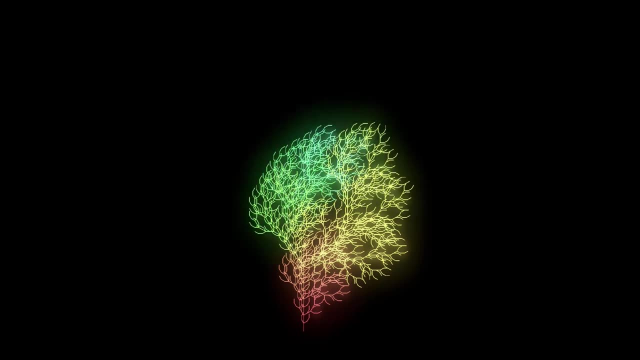 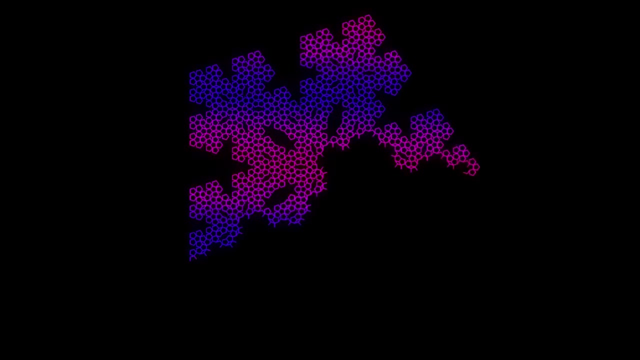 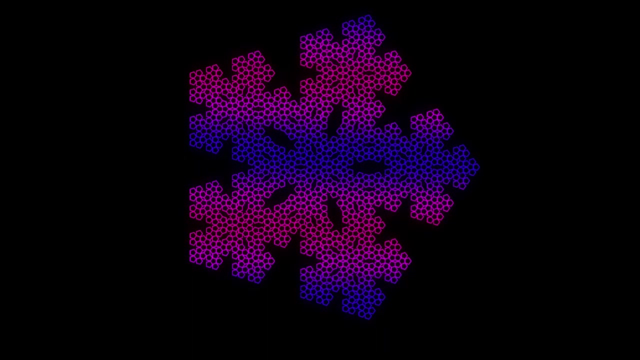 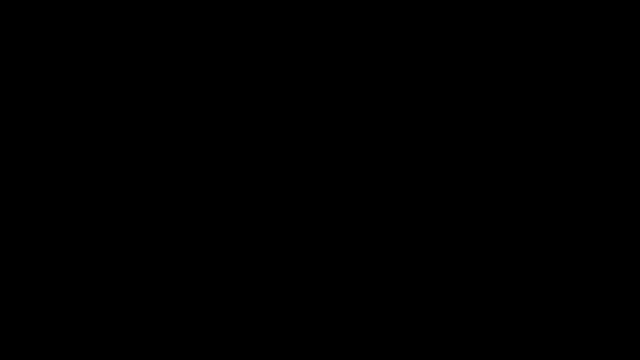 Yes, Yes, Yes, Yes, Yes, Thank you. From there on, I wanted to try out a different type of fractal. My goal was to visualize the Mandelbrot set. The idea behind it is not that difficult. Let's consider a plane like your screen, for example. 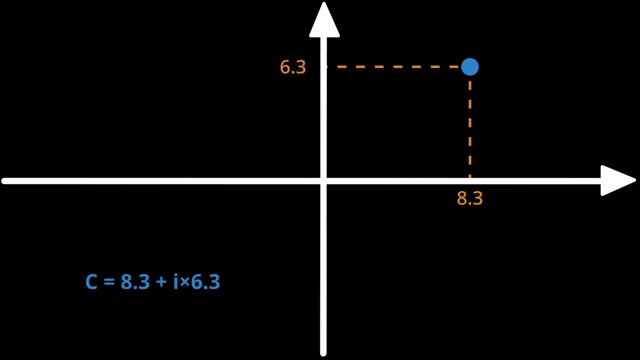 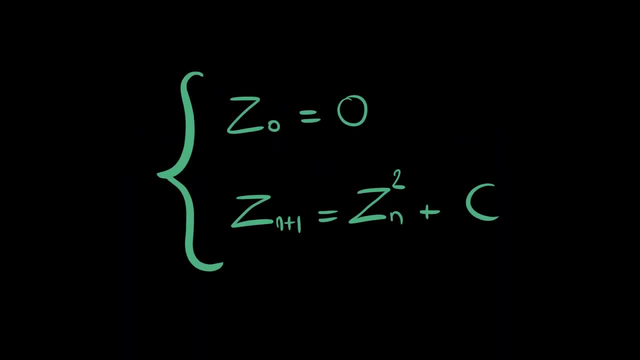 We can assign a value to each point depending on its position on each axis. Then we compute this sequence Which at each step gives another point in the plane. For example, with this point we have this sequence which goes to 0.. 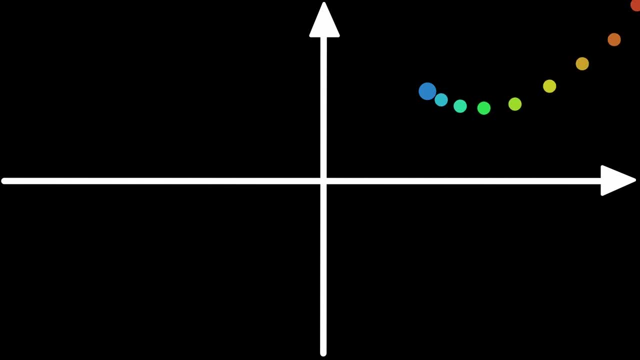 And with this point the sequence will go really far away. So we say it trends to infinity. An interesting fact about this sequence is that if a point goes further than this ring, we can be sure that the sequence will tend to infinity. 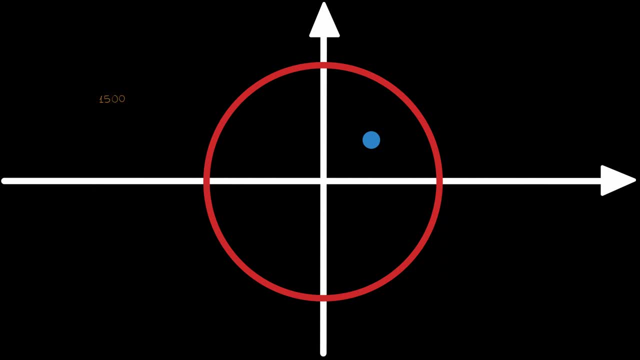 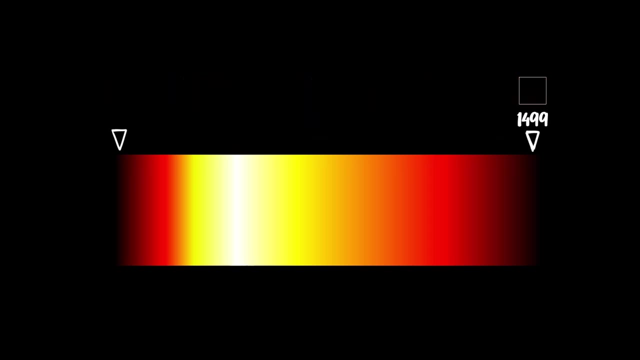 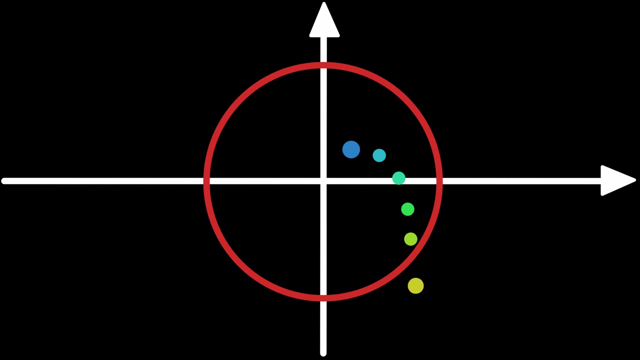 So we can take a point and compute the 1500 first values of the sequence And, based on when the point goes further than the circle, we can assign a color to it. For example, the sequence for this point goes behind the ring at value number 5.. 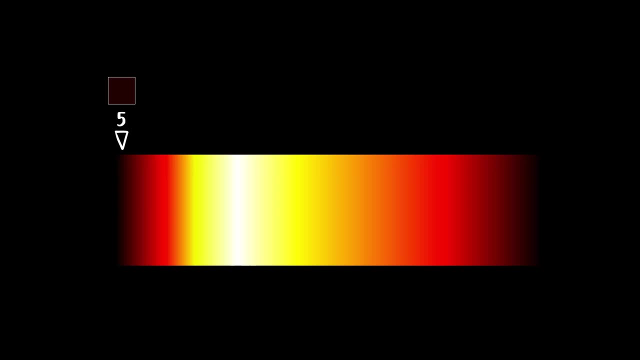 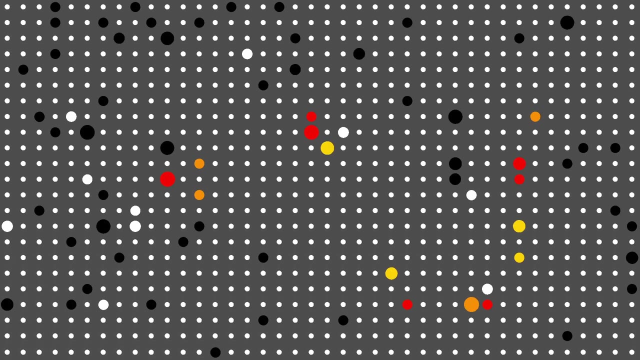 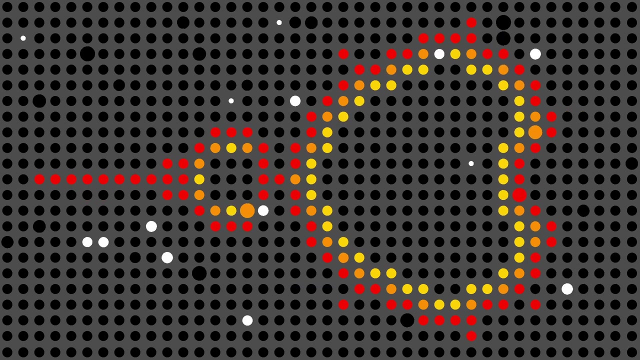 So it will get this color Great. Now, if we consider each pixel on the screen, we can compute its color, But this will take a lot of time as it implies to compute 1920 times 1080 sequences, each up to 1500 values. 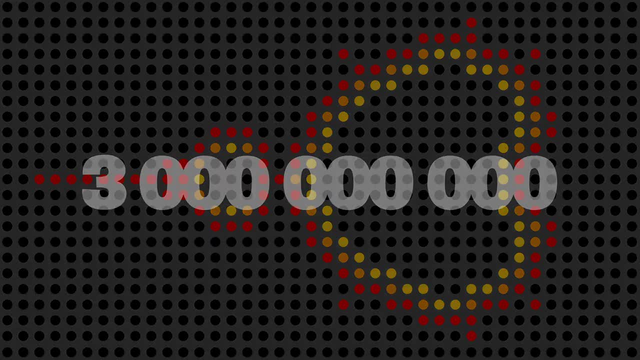 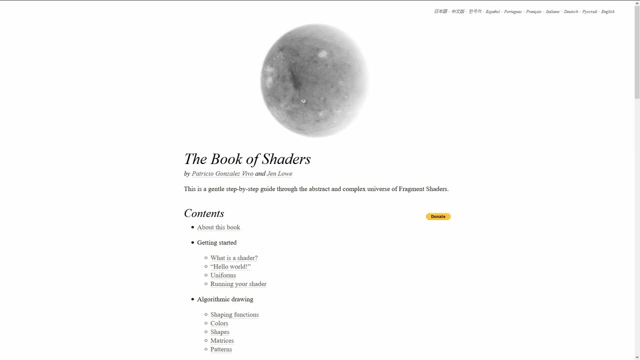 This represents more than 1,000 pixels. This represents more than 1,000 pixels. This represents more than 3 billion operations. As explained in the book of shaders, the processor is good to compute complex things, but terrible at computing a bunch of smaller ones. 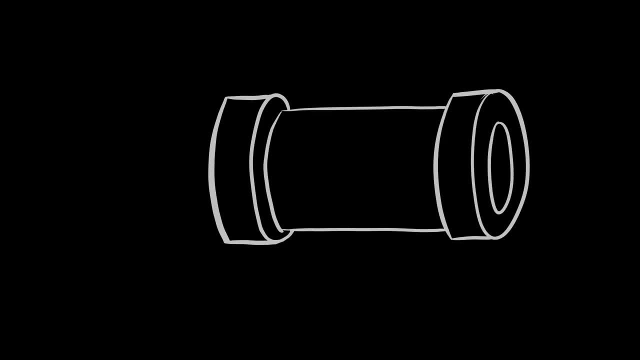 You can visualize it as a big pipe where only one task can enter at the time. What's needed is parallel processing- Many small pipes running in parallel- And we have it. We have this in the Graphic Processor Unit, which is in your graphic card. 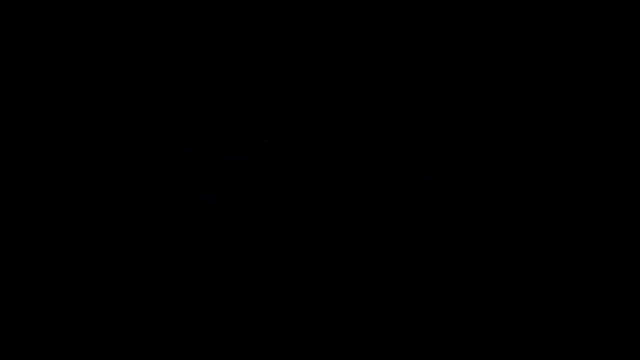 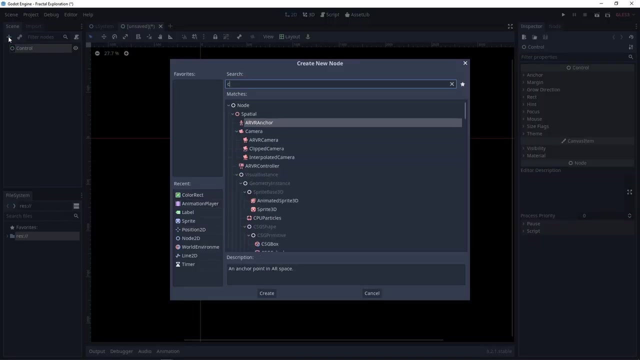 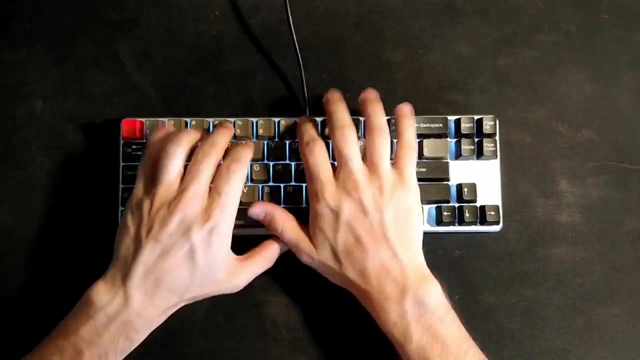 In order to communicate with it. we will use a pixel shader. It is quite easy to do in Godot. I have created a new scene, added a color rect node and attached a new shader as material. Then I wrote down some code and here is the result. 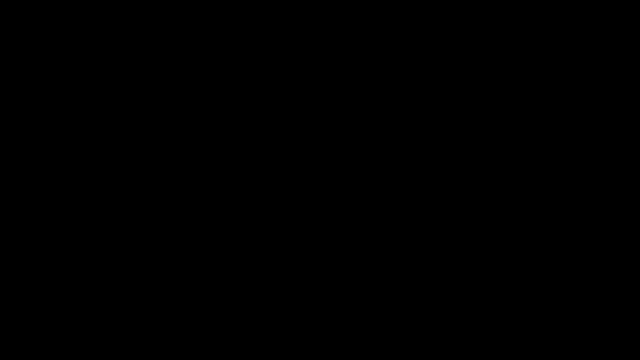 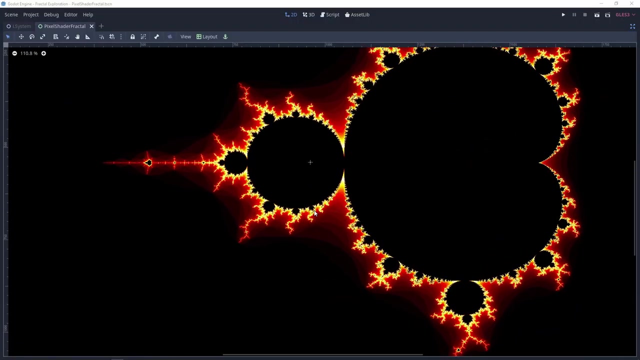 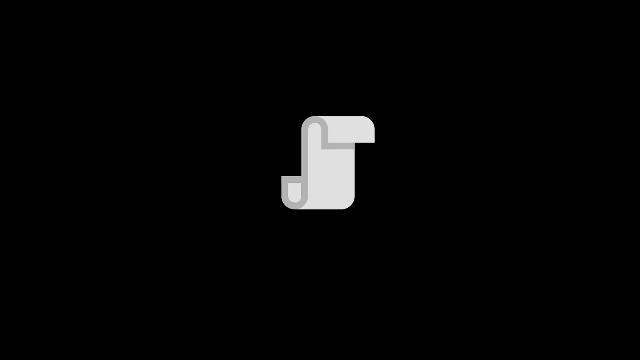 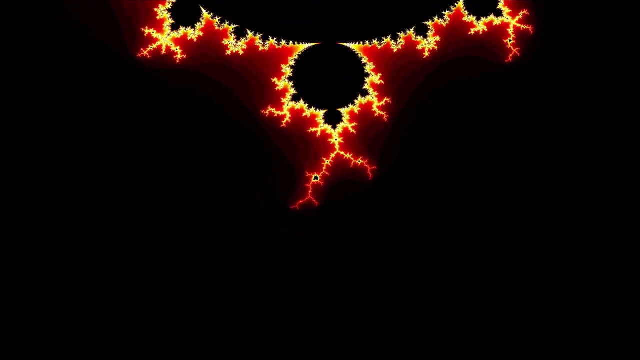 I think it looks really good, So I added a center point variable and a scale variable. As it is a shader, we can of course, zoom on it without pixelization. So I added a script with a zoom and it was slow, so I made this zoom exponential, which is a lot faster. 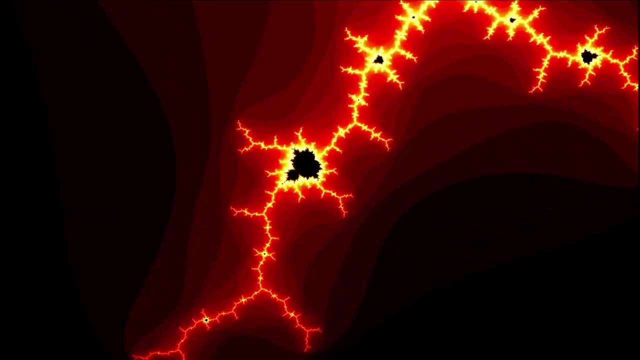 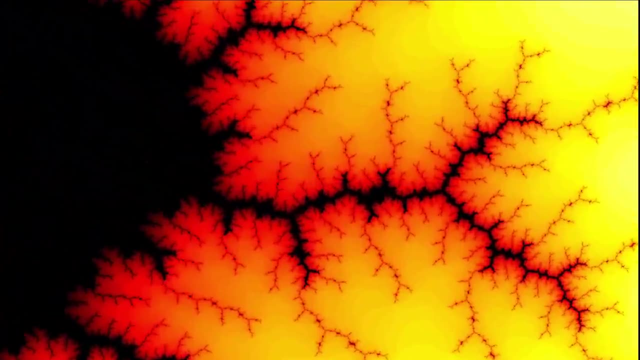 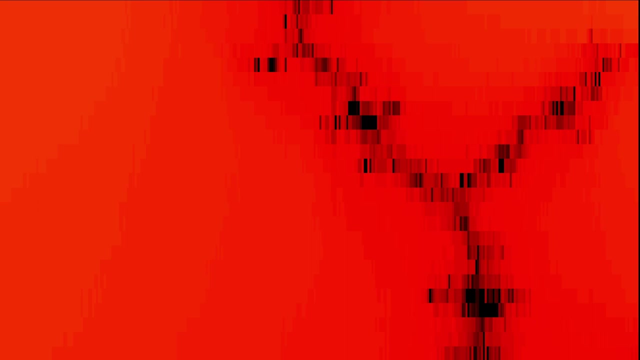 If you flash it, you get a much smoother view. This is looking crazy, Yo, What the fu-? Ok, so I searched on Google. what was the issue? In fact, this is due to the precision of my variables and operations. Basically, we zoomed so much. the points here are so close. 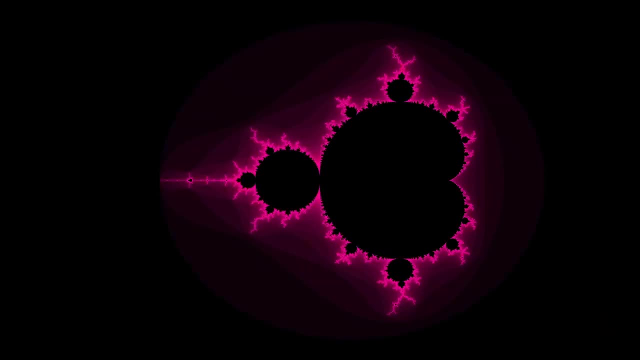 the computer think it's real, So it takes the same time to zoom. It takes time to open the words and say so. thinks they are equal. I know it is possible to do even more and create some crazy zoom, but I prefer to leave this out for the moment. If any of you intelligent guys want to suggest. 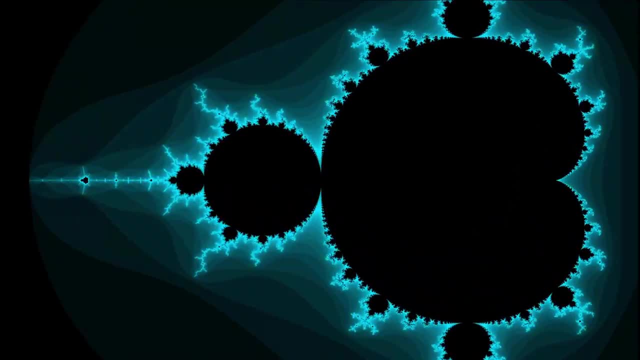 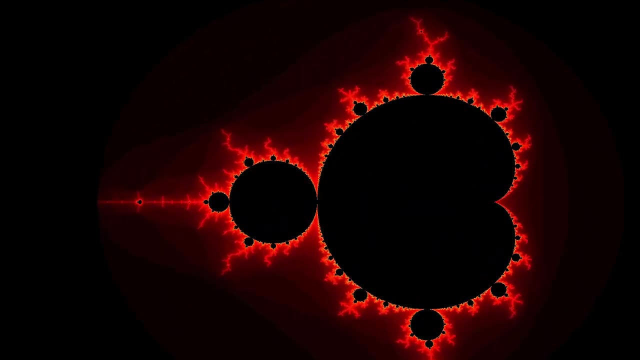 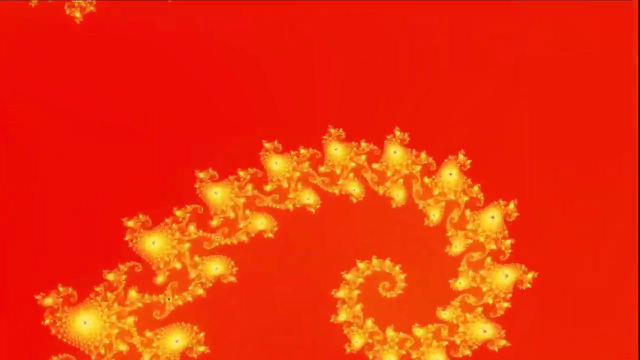 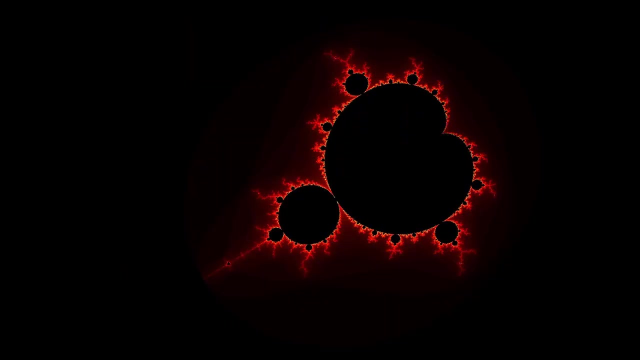 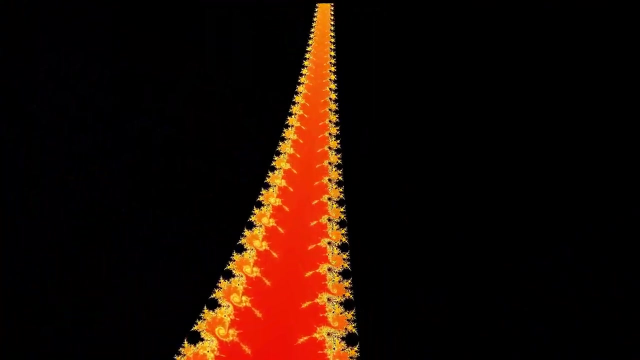 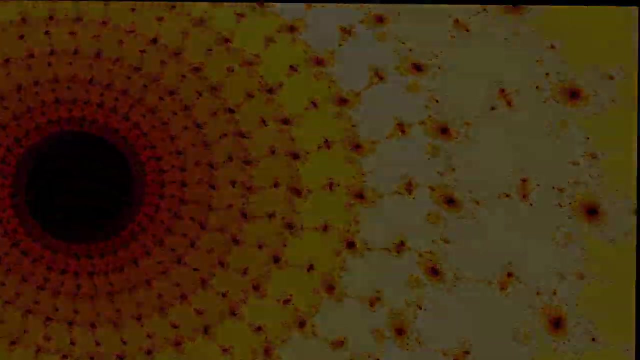 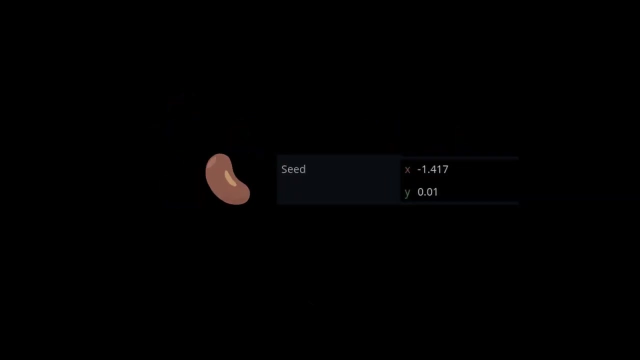 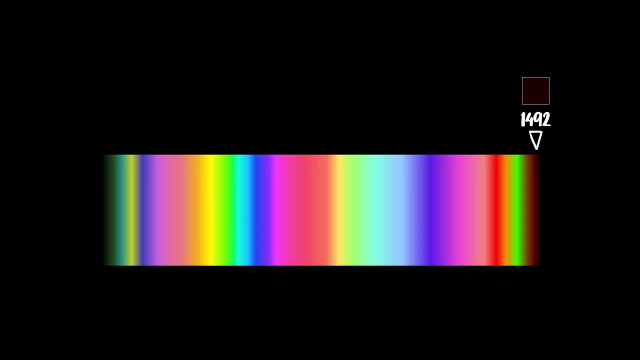 an improvement in the comments. you're welcome. Then I wanted to visualize the Julia set. It is almost the same, except it depends on a seed. I have set up a crazy gradient like so, And there we have it. If I change the seed, the